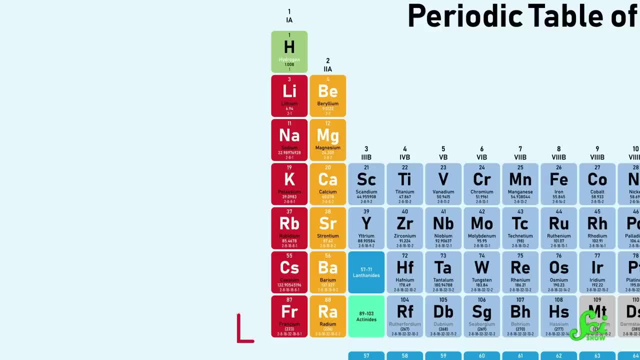 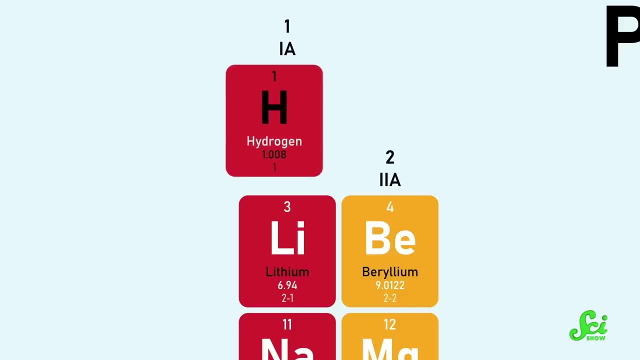 It's probably sitting up above lithium at the top of the alkali metals. But look a little closer. Maybe it's shaded a different color than the elements below it. Maybe it's floating a slight distance away with a little drop shadow. It looks like it's embarrassed to be there, like it's not really with those guys. 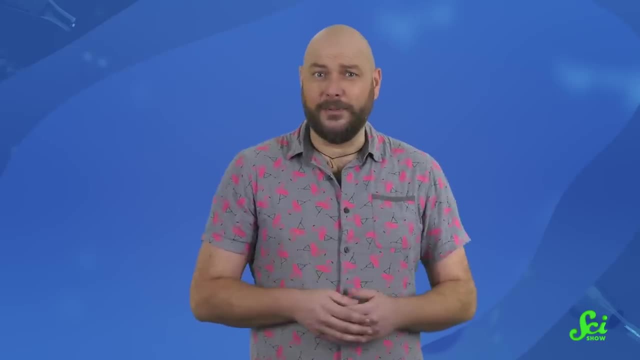 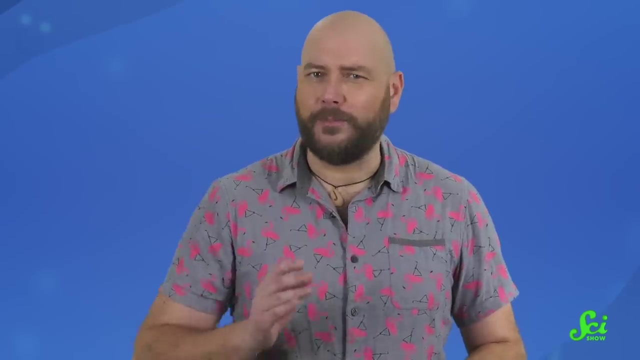 This isn't a graphic design mistake, Even though it's the simplest element. chemists actually don't agree on where hydrogen belongs in the periodic table. There are at least three credible places you can stick it, and that's a problem for our understanding of how elements work. 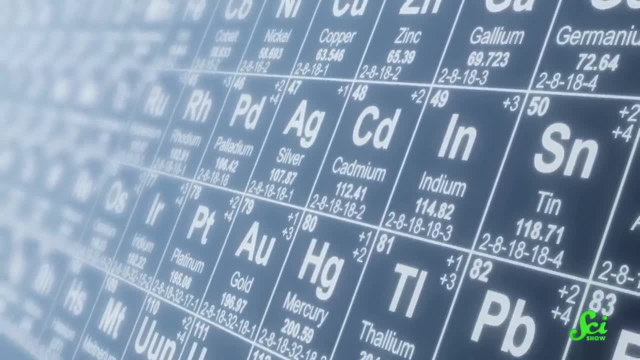 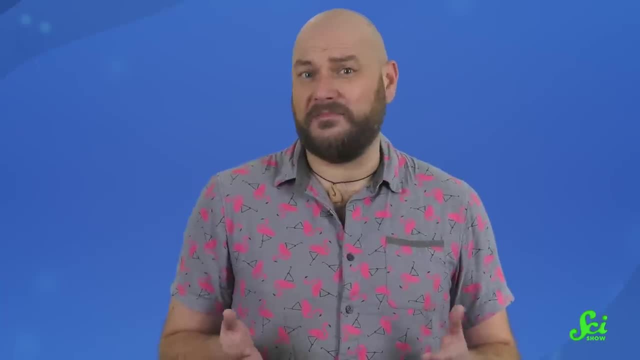 As fixed and immutable as it may seem, hanging on your high school chemistry classroom wall, the periodic table is not a problem. The atomic table is really a work in progress. It does a lot of things we like because they make sense. Elements are listed in order of ascending atomic number. 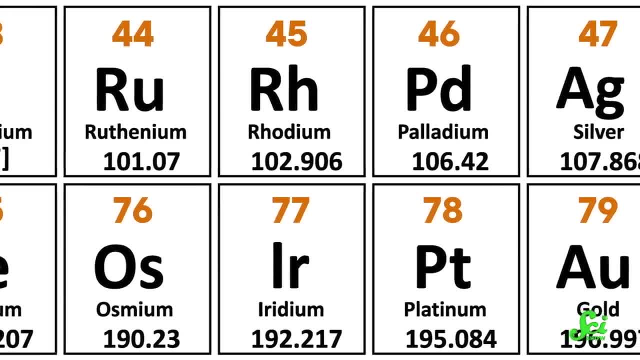 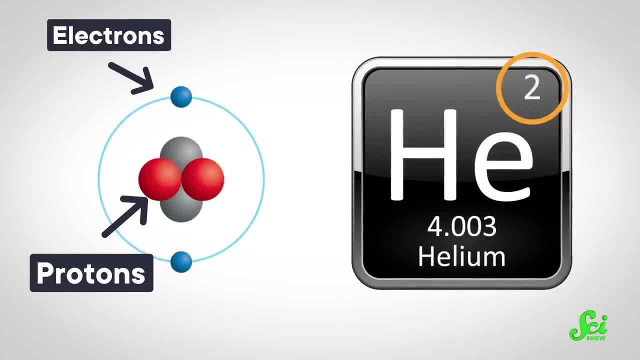 And that's not just for the sake of making a tidy list. It's related to their chemical properties. Atomic number represents the number of protons an atom has, but also the number of electrons, And the reason for this would require us to go into quantum mechanics. 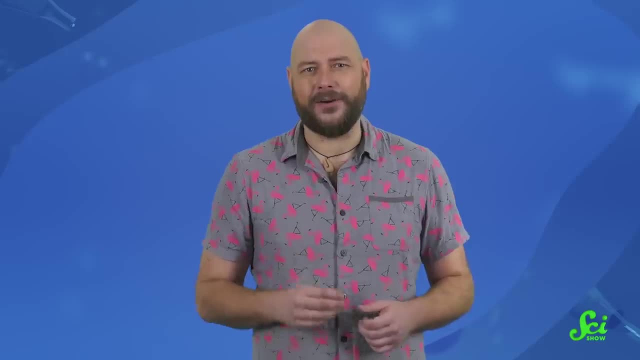 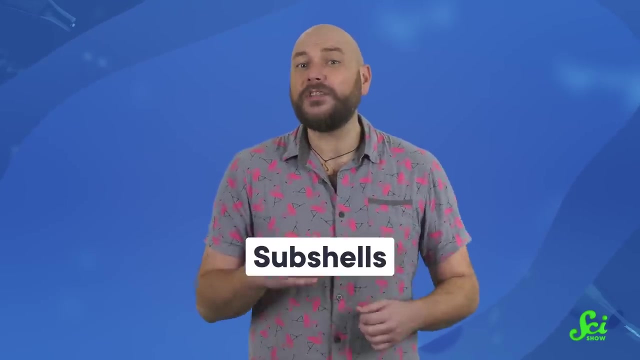 But electrons will always fill up in specific patterns. After a while the pattern starts over again. This is because the electrons are going into specific subshells, which are like distributions of energy around the atom. When those subshells fill up, the pattern repeats in new subshells. 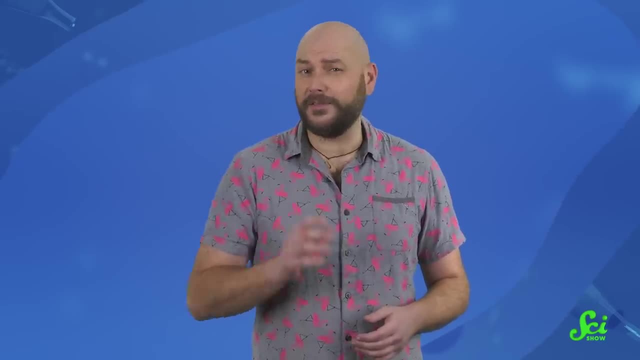 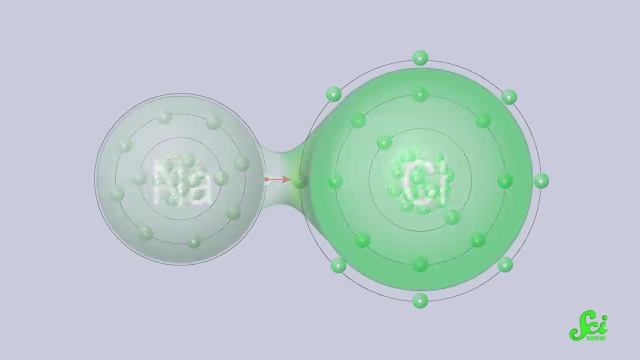 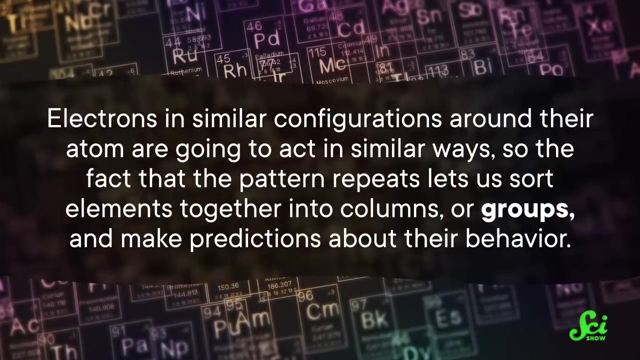 Which means that by listing the elements in order, something interesting happens. Electrons are everything in chemistry. All chemical reactions are just electrons swapping places until you get down to the nuclear stuff that is. And electrons in similar configurations around their atom are going to act in similar ways. 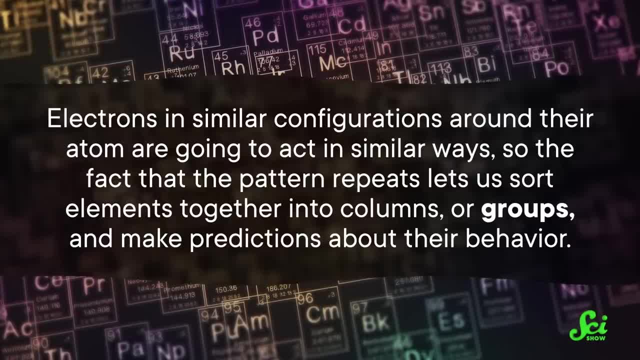 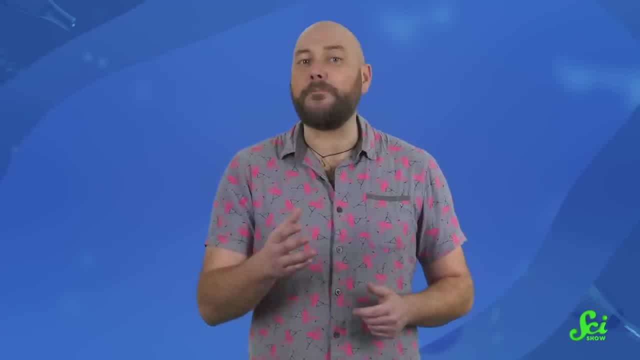 So the fact that the pattern repeats lets us sort elements together into columns or groups and make predictions about their behavior. These repeating properties are that periodic thing in the name Lithium and sodium. both have only one electron in their outermost subshell. 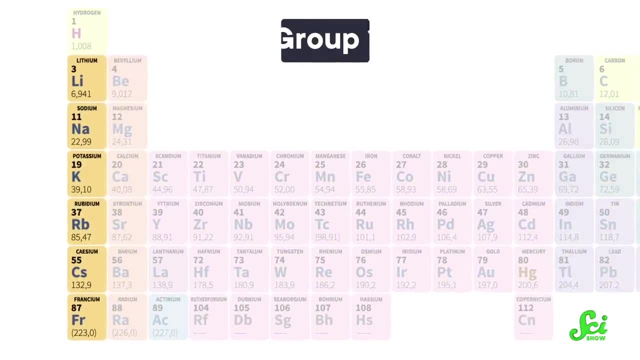 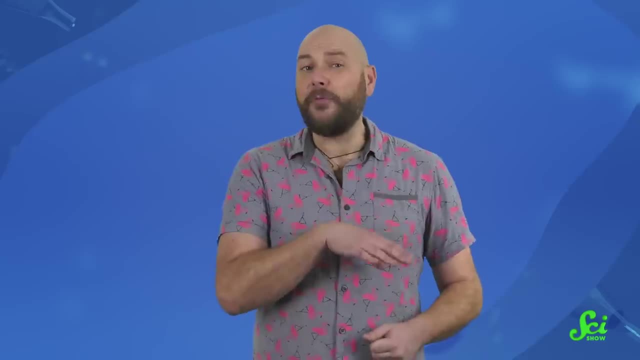 They react in similar ways, so we put them in the same group, group one, Which makes it really annoying that the very simplest element flouts these periodic rules. It both does and doesn't act like at least three different groups and doesn't really fit in with any of them. 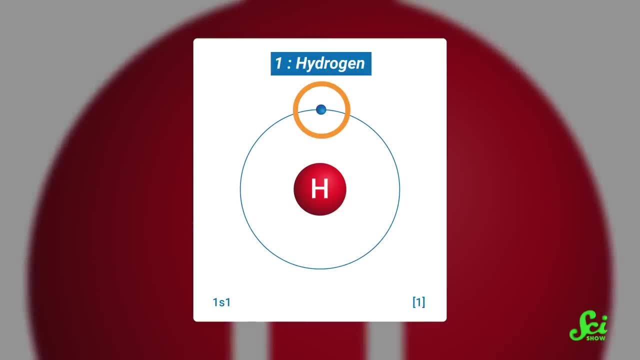 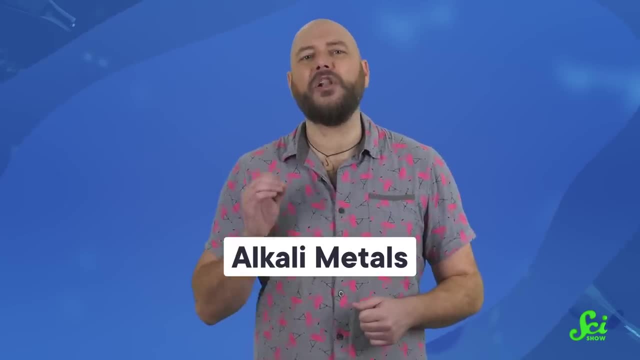 Hydrogen has one lone electron in a shell that has room for a total of two. That makes it resemble the alkali metals like lithium and sodium, because they all have a lone outer electron, But also like group 14,, which starts with carbon, which have their outer shell half full. 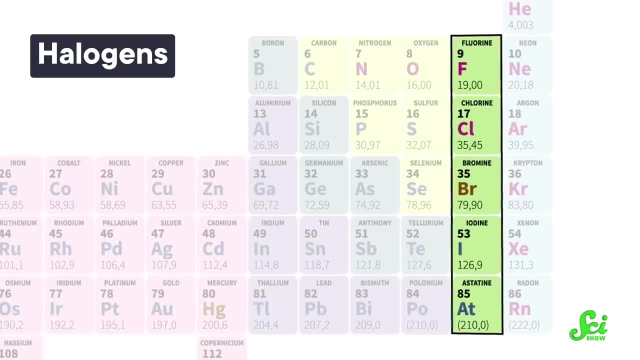 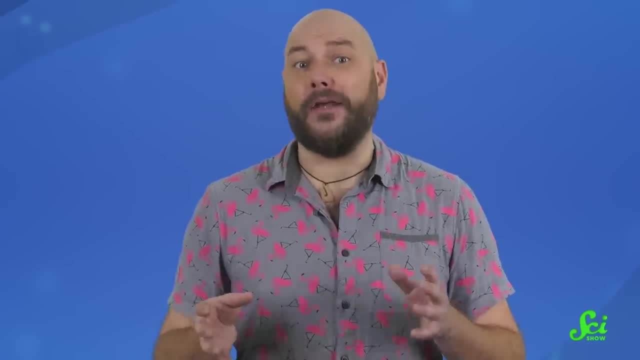 But also also the halogens, starting with fluorine, because they have room for one more electron. Let's quickly look at what makes each of these options both right and wrong. First, the alkali metals, which is where you usually see hydrogen. 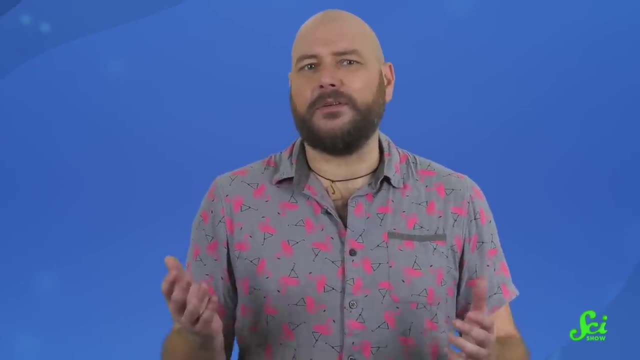 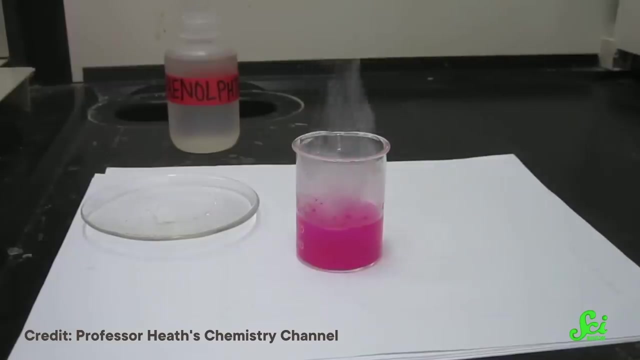 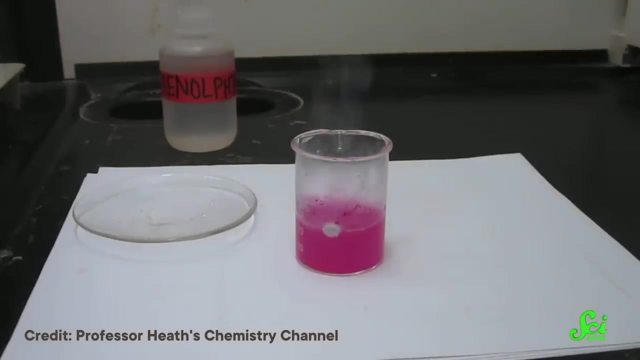 Less because it's the best option and more because chemists sort of gave up arguing with the graphic designers, not with other chemists. If you had a good chemistry teacher, they probably took out a lump of lithium or sodium and let you watch it sputter around a beaker, literally catching fire in contact with water. 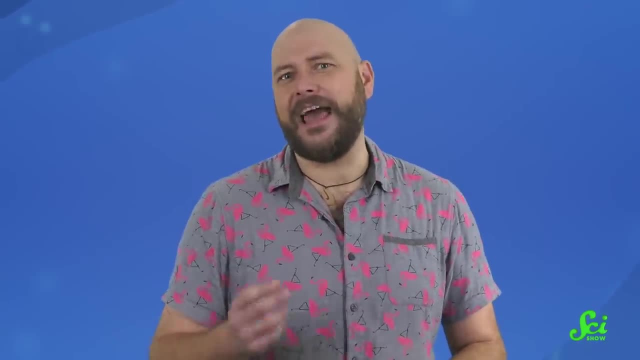 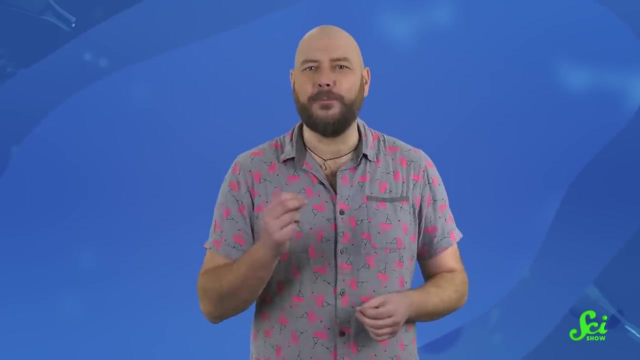 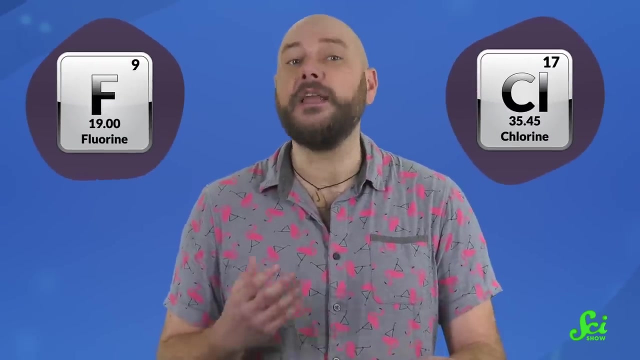 While hydrogen doesn't do that, it does behave like the alkali metals in some ways. All of them tend to lose that one outermost electron to form an ion with a single positive charge, H+, Na+. They also tend to react with similar partners like fluorine and chlorine. But there are differences. Hydrogen, you may have noticed, is not a metal. Some really intrepid chemists say they've convinced it to act like one under extreme circumstances, which would be an argument for it being an alkali metal, But not everyone agrees that counts. Hydrogen also tends to lose that one outermost electron to form an ion with a single positive charge: H+, Na+. Hydrogen tends to form really different compounds, even when it's bonding with the same thing as an alkali metal. Hydrogen chloride is a corrosive gas. 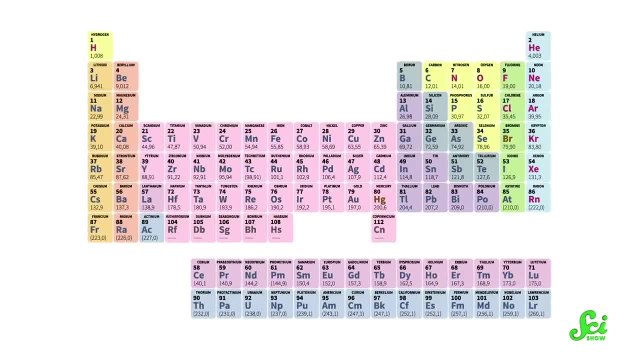 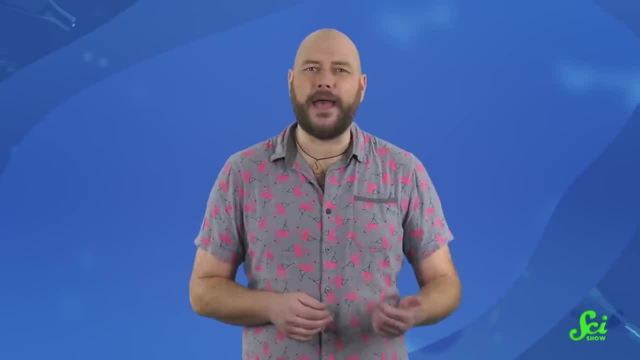 Sodium chloride tastes great on your fries. Speaking of chlorine, let's skip ahead to the halogens. Fluorine chlorine on down, Because hydrogen also forms similar ions to the halogens. You can get hydrogen to gain an electron and make a hydride ion, H-. 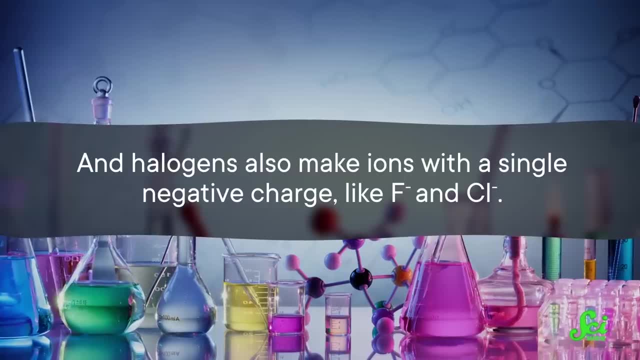 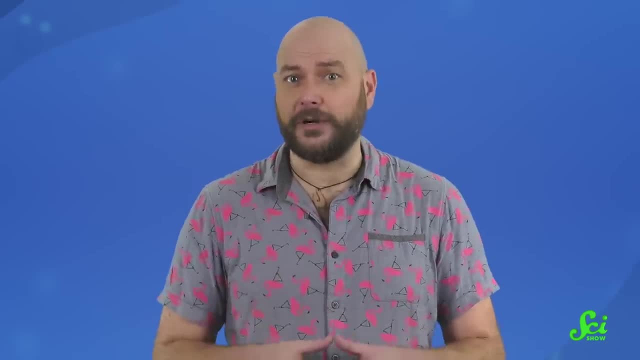 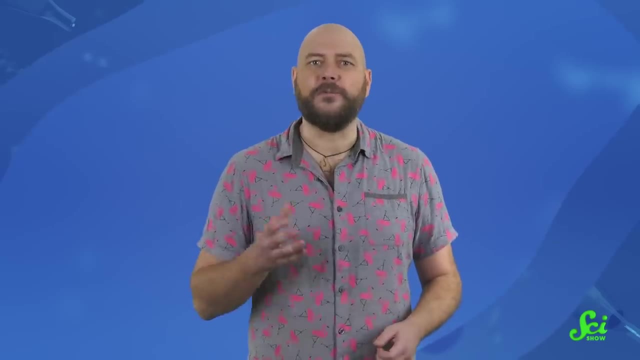 And halogens also make ions with a single negative charge, like F- and Cl-. Hydrogen, fluorine and chlorine also all make gases at room temperature and all exist in diatomic form, H2F2.. On the other hand, hydrogen differs from fluorine in a big way. 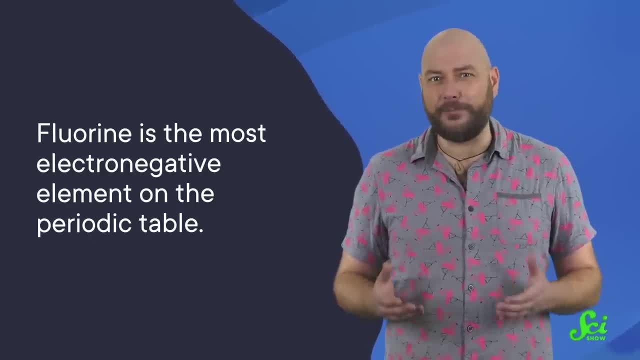 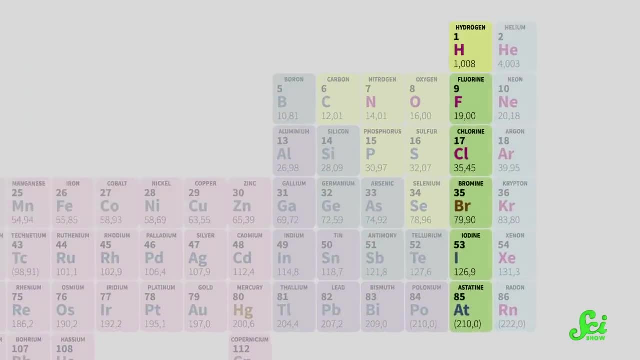 in that fluorine is the most electronegative element on the periodic table, meaning the greediest and most likely to hog electrons from its bonding partners. If hydrogen were placed above fluorine, you'd expect it to be even more electronegative. 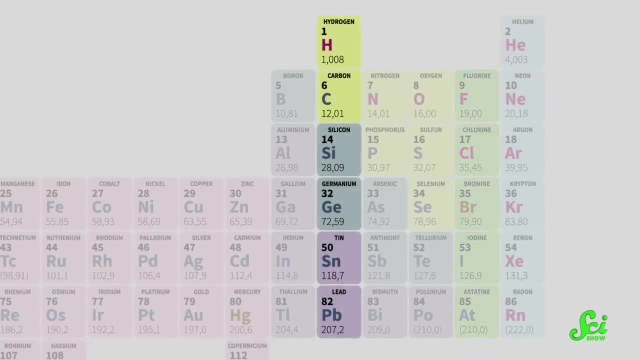 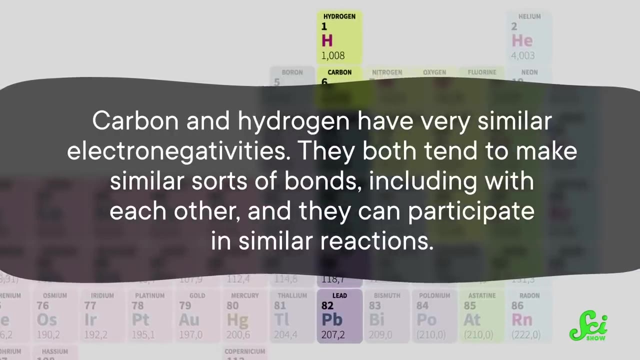 but it's actually much better at sharing. That brings us back to group 14, the carbon group. Carbon and hydrogen have very similar electronegativities. They both tend to make similar sorts of bonds, including with each other, and they can participate in similar reactions. 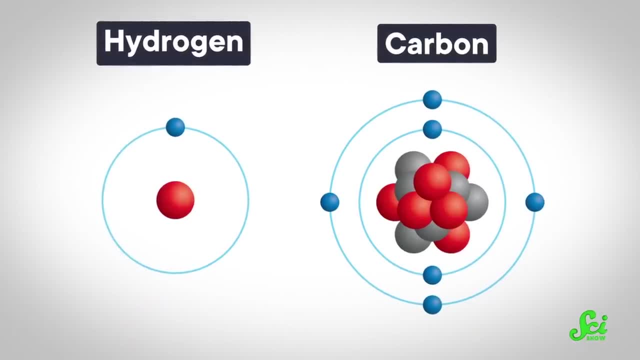 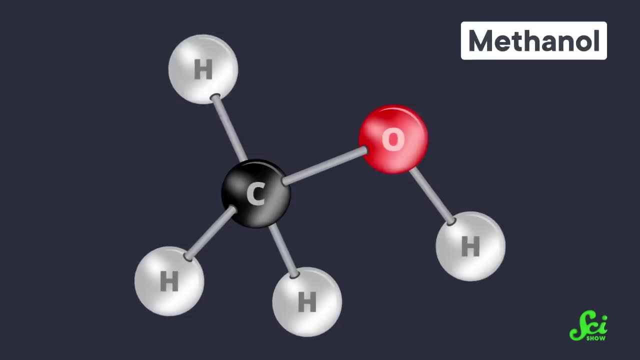 But some people will step back and say that comparing an element with one outer electron to one with four just isn't actually the same thing at all. Like carbon, has this amazing habit of linking hands and making bonds at once that you don't see with hydrogen. 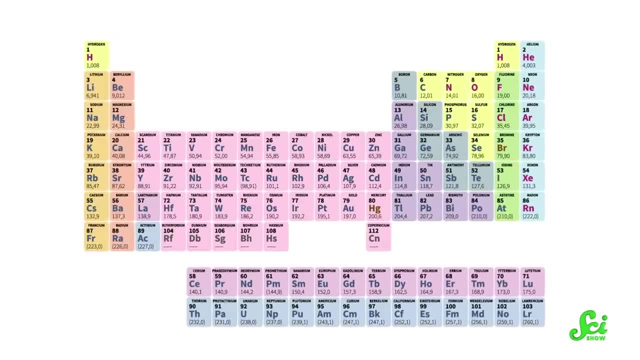 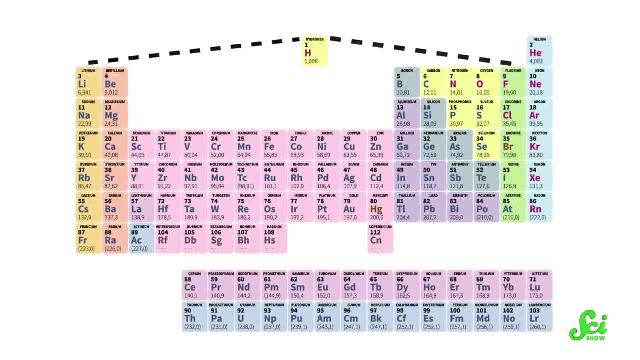 So there just isn't a clear, right answer. Hail Mary. proposals include putting it with both the halogens and the alkali metals, or sort of linked to them with dotted lines, or giving up and hucking it somewhere in the middle. I don't think this argument is going to end any time soon. 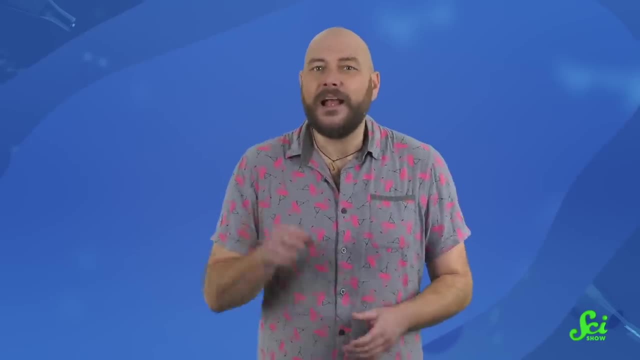 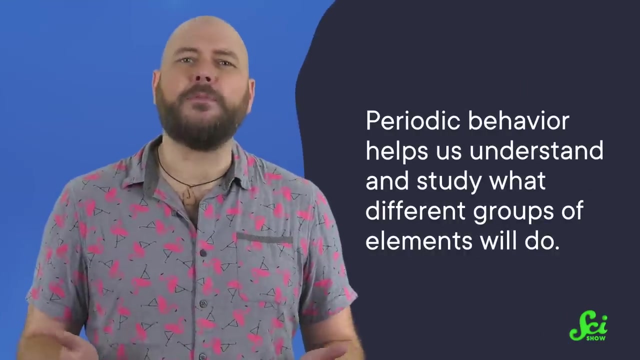 And this isn't just some abstract squabble between chemists. That periodic table was on your classroom wall for a reason: It's a predictive tool. Periodic behavior helps us understand and study what different groups of elements will do, And a well-constructed table will help you learn those properties. 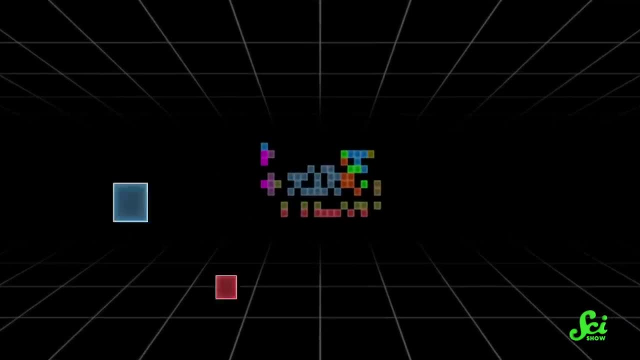 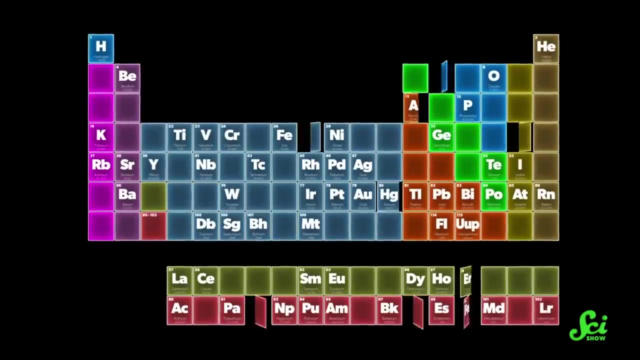 and make predictions about how elements will behave. whether it's a teacher asking you the electronegativity of boron or a chemist trying to work out the ionization energy of dubnium, If an element is in the wrong place, you'll end up making wrong predictions. 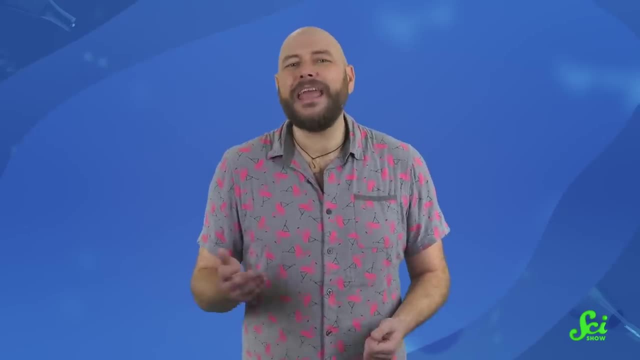 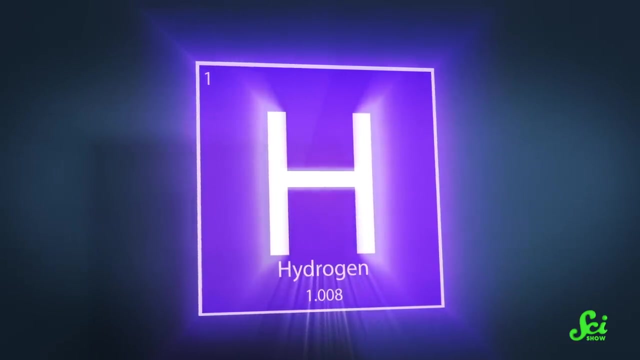 And if you give up and don't put hydrogen anywhere, you can't predict anything at all. In the end, no one's going to get through any study of chemistry without learning that hydrogen is unique and has some properties you just can't predict. 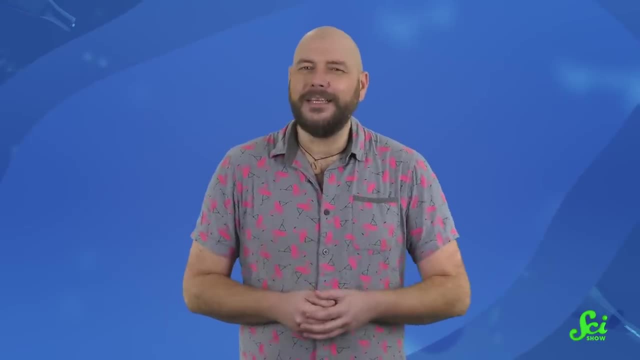 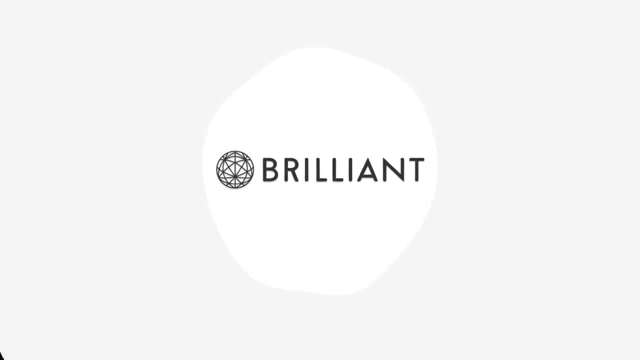 So maybe we should tell it to stop being so embarrassed. It's just special Chemicals are awesome. Put two of them together and you've got a compound or a molecule. For more chemistry, basics and molecular mischief, you can take the brilliant course: all about molecules. 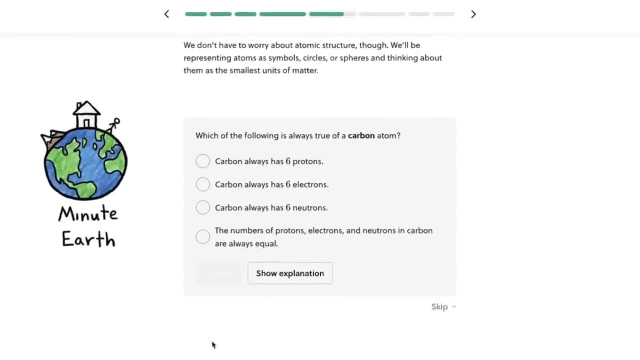 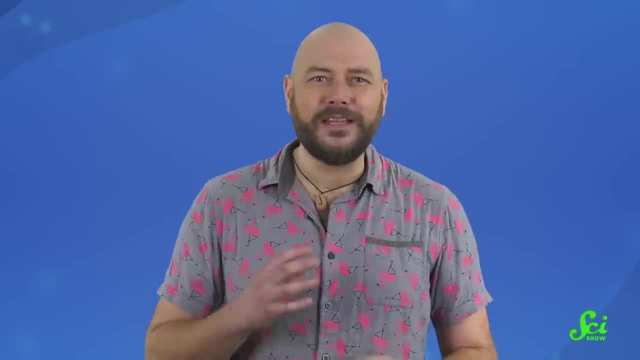 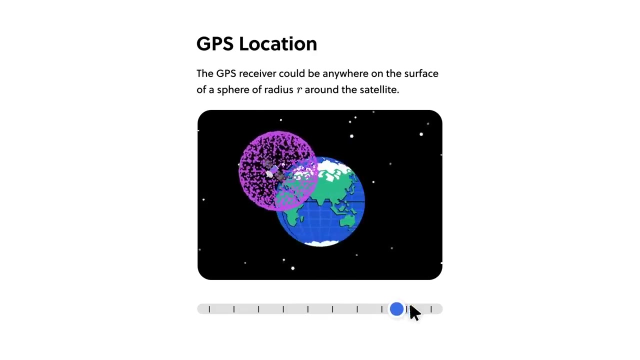 This course was made in collaboration with another YouTube channel, MinuteEarth, And, as you know, there are some really good science communicators on YouTube. But the partnership is what really sets this course apart, Because Brilliant makes online learning interactive with thousands of lessons in science, computer science and math. 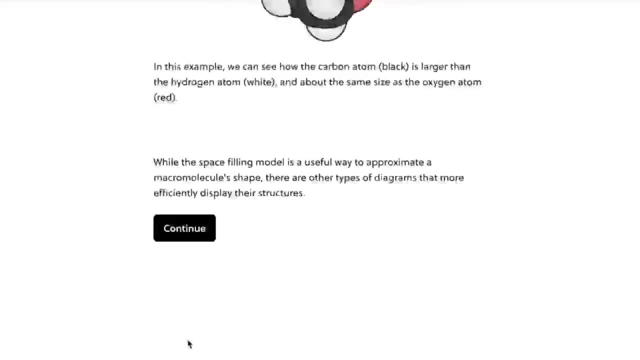 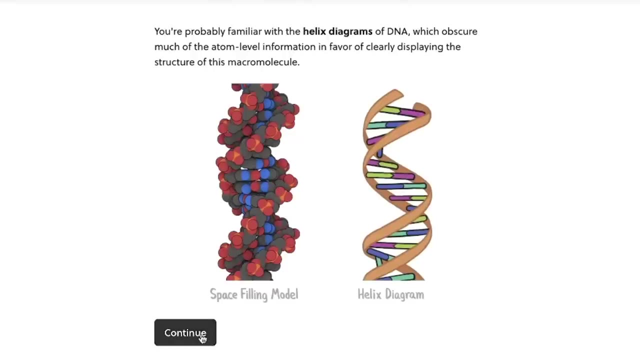 At the end of this particular Brilliant course, you'll know what different molecules are just by looking at their diagrams And real learning like this makes us proud to have Brilliant supporting this SciShow video. To try Brilliant with your first 30 days free. 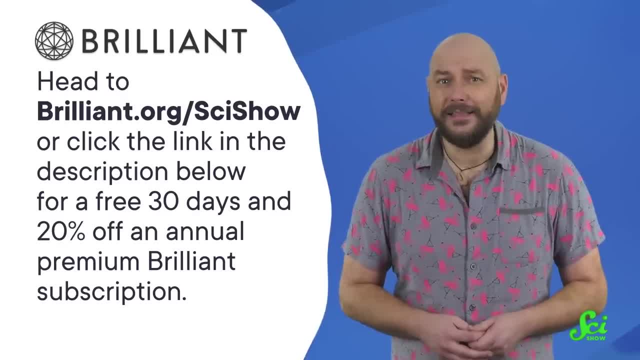 you can go to Brilliantorg slash SciShow or click the link in the description below. That link also gives you 20% off an annual Premium Brilliant subscription. Thanks for watching. 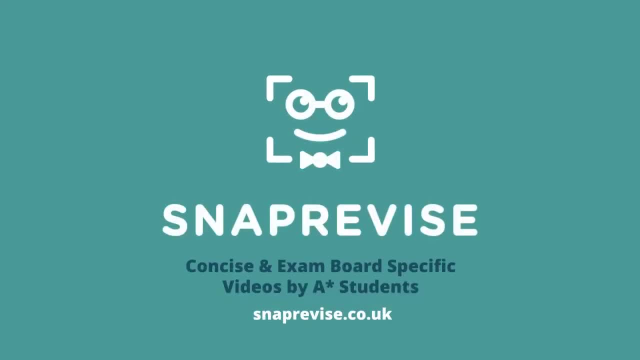 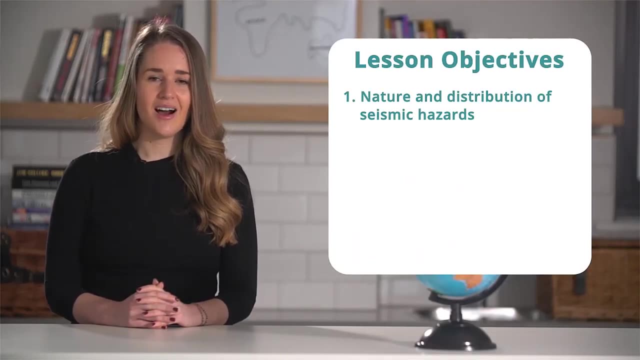 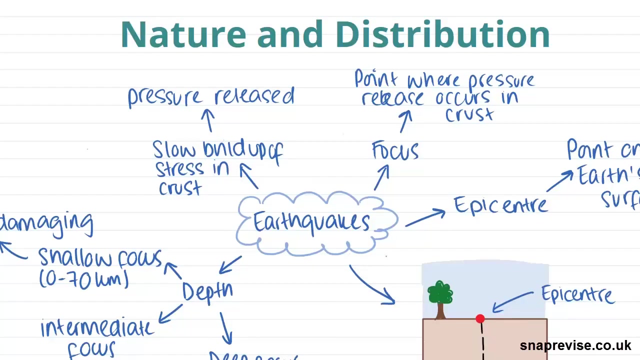 Hi guys, In this video we will be learning about the nature and distribution of seismic hazards, understanding their magnitude and frequency, and the impacts and management of these events. So firstly, we're going to look at the nature of seismic hazards. So seismic hazards, as I 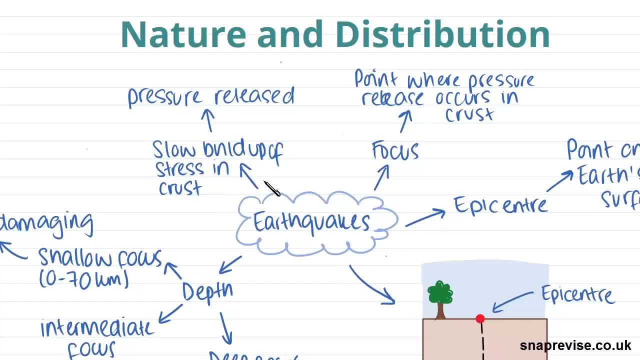 mentioned before are earthquakes, and they occur when there is a slow buildup of stress in the crust, and when this pressure is finally released, it causes an earthquake and this tends to shake the ground. So this often happens at conservative plate boundaries, and this is when the plates are. 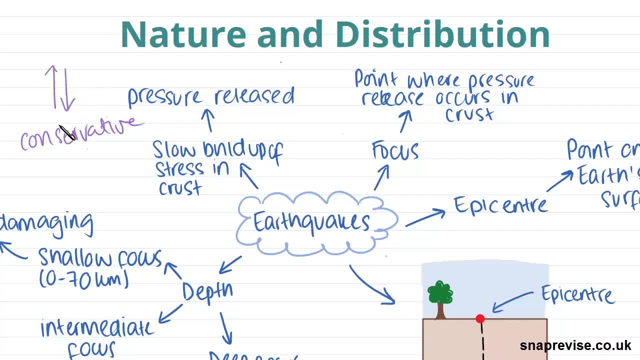 moving in opposite but parallel directions to each other like this, and often the plates can get stuck in each other and this is when the stress builds up. but I'm going to look into the formation of earthquakes in more detail later on. So two main things that can happen. 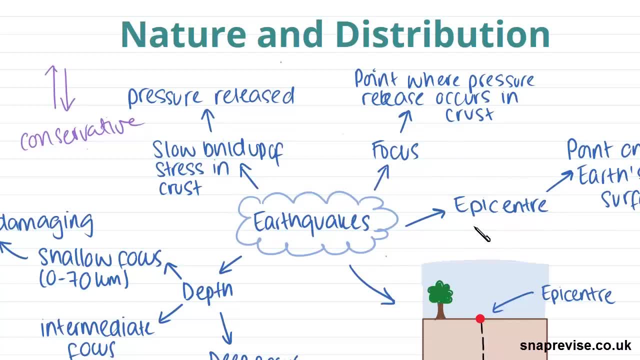 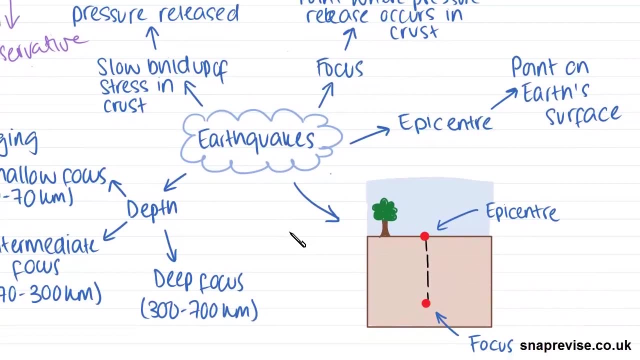 when an earthquake occurs. So one of the things we need to know about earthquakes is what is the focus and what is the epicenter? So the focus is the point where this pressure release occurs in the crust, and you can see this on this diagram. here The focus is the specific point in the crust where the earthquake originates. 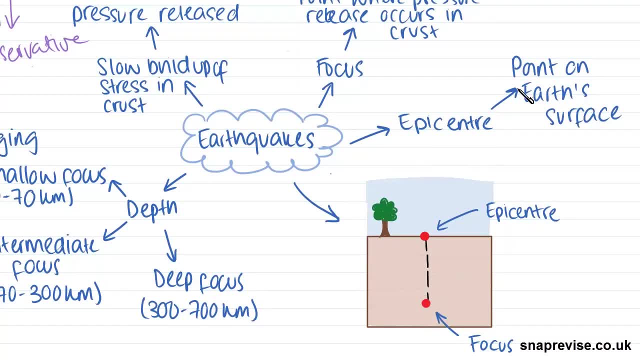 from, whereas the epicenter is the point on the earth's surface. So this is going to be the point directly above the focus, but on the actual earth's surface, and this is often where we refer to as being location of an earthquake, when one occurs. So, alongside this, earthquakes can happen at different depths, which are shallow, intermediate and deep. So shallow earthquakes are the most damaging earthquakes because they're nearer the surface. therefore, when the earthquake waves reach the surface, they are at their most powerful and these occur at zero to 70 km deep. Intermediate are a bit less powerful and half as powerful.